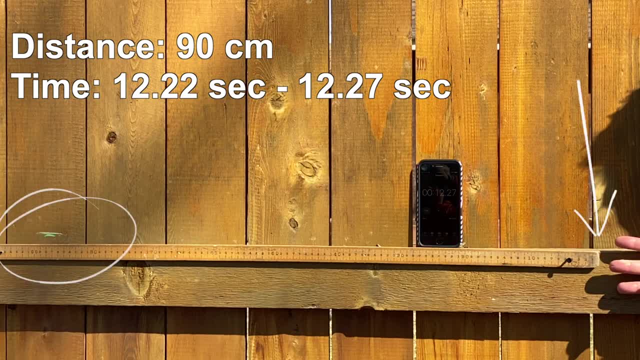 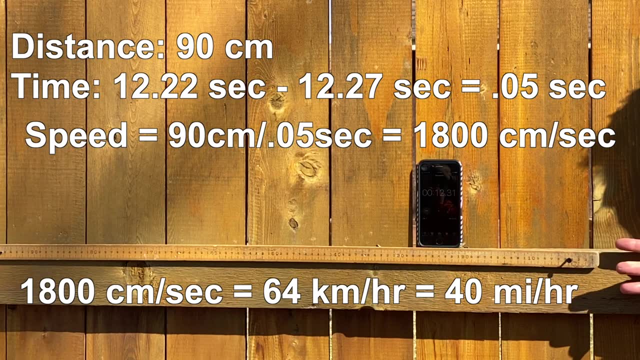 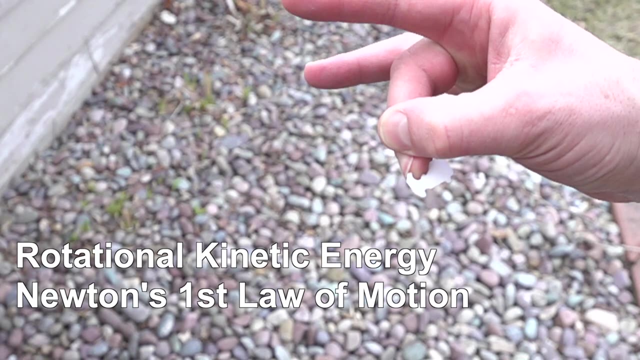 of an object So we can see when it crosses the zero mark. it's, at time, 12.22 seconds. It crosses the 90 centimeter mark, or 12.27 seconds. And we've got 90 centimeters. That's 40 miles per hour, That's 64 kilometers per hour. How we getting those kinds of speeds? 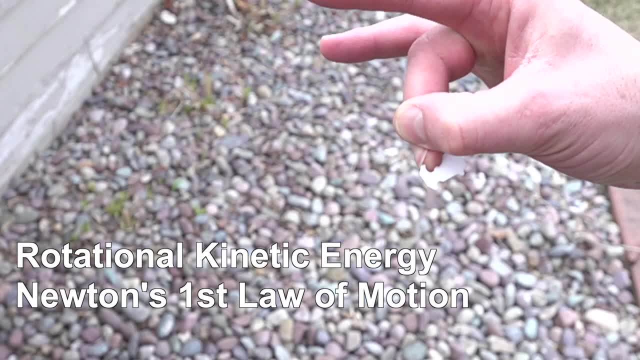 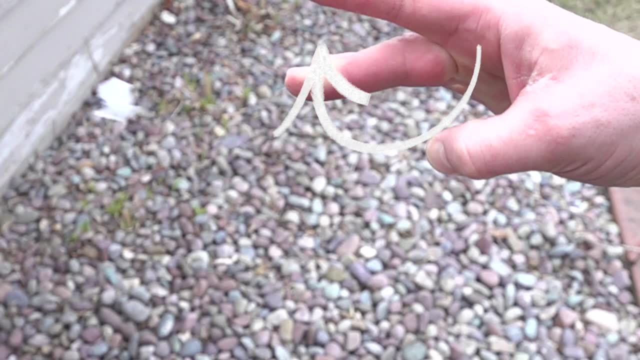 Well, it has to do with rotational kinetic energy. When my finger comes flying off my thumb, it's providing energy or affection force. that goes with the clip. Now the clip would just stop with my finger. but Newton's first law says an object will remain in motion unless acted on by an outside force. and since there's no outside, 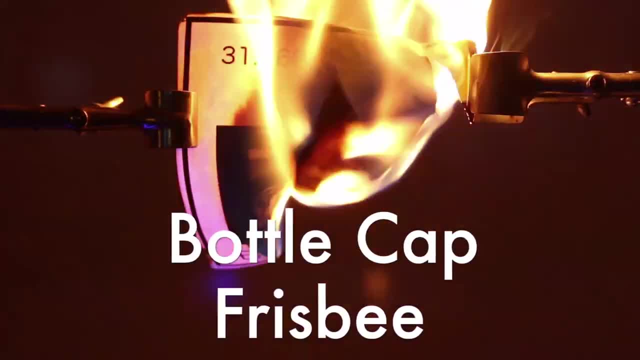 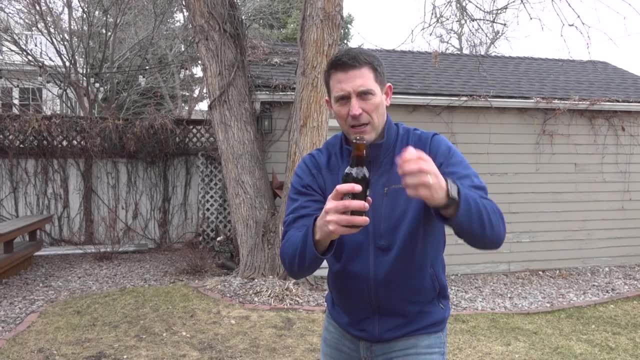 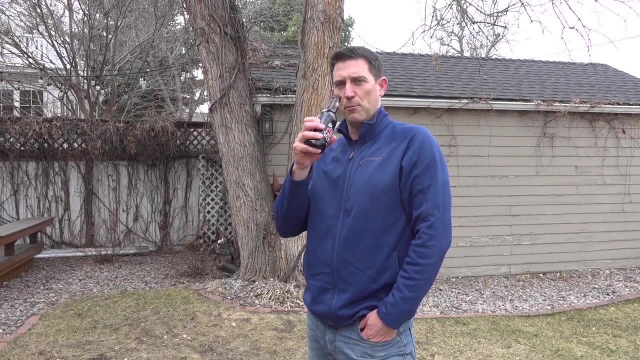 force it keeps going. I'm going to show you a handy dandy trick. Got all these people running around with these bottle openers on their hands so that they can open up bottles these days. You thought it was to show a sign of marriage, but turns out it's just a bottle opener. 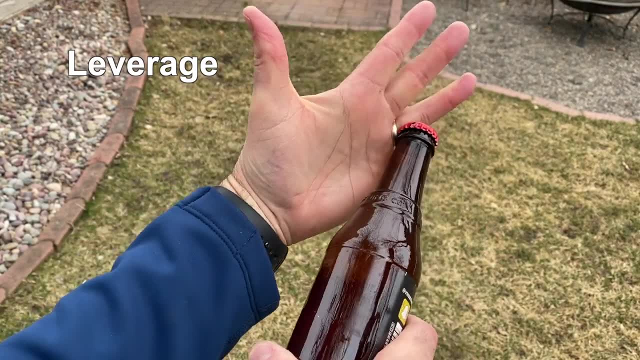 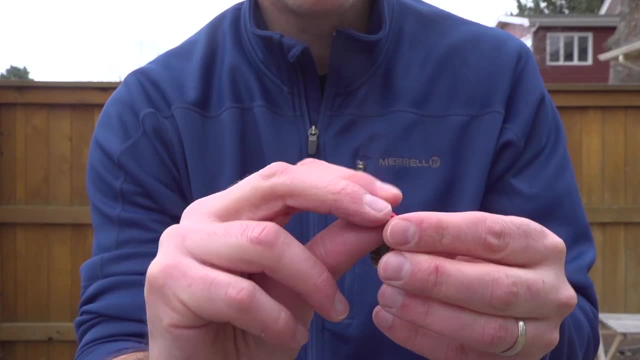 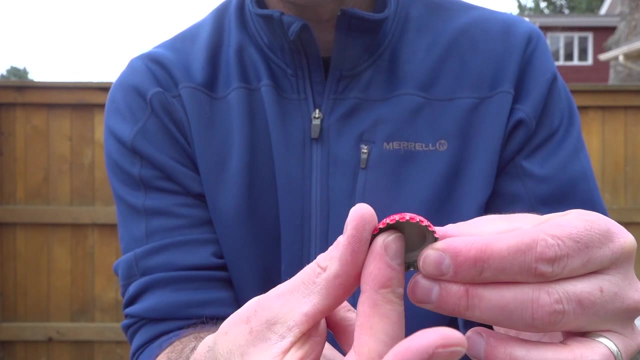 The reason this works is also explained by physics. This is just leverage, so I'm using my finger and then the ring as a lever to pry something open. To get it to fly, I've got to hold it in a very specific way. Basically, I'll be snapping my fingers and then I'll just have the 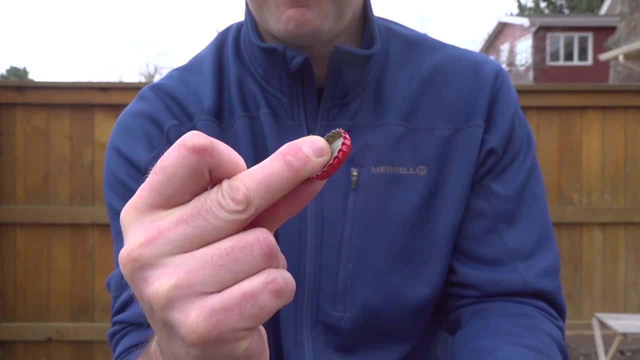 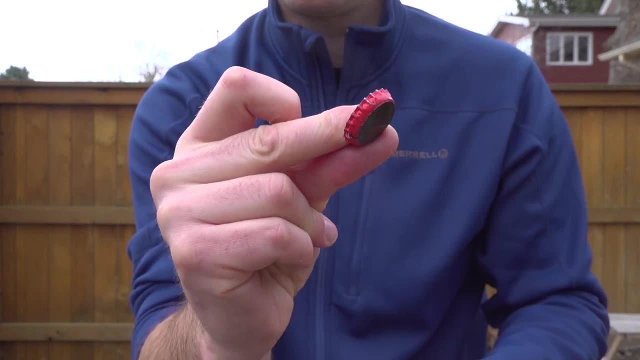 bottle cap in between my snapped fingers. That provides the rotation, the energy, the rotational motion to get it to fly off my fingers. And, as you can see, I've got a little bit of a problem here. I've got a little bit of a problem. 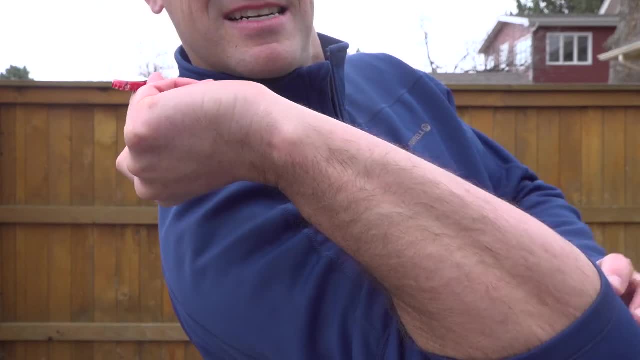 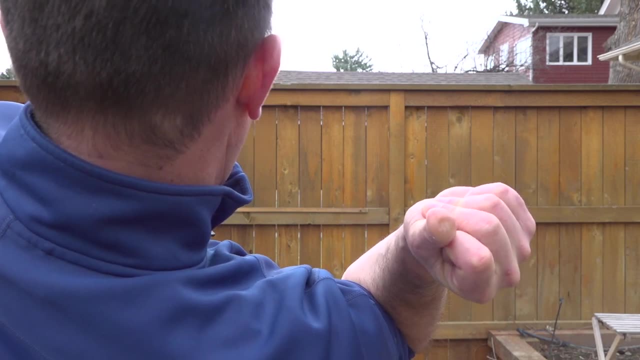 here. As you can see, it travels along the path of my forearm, so if I want to shoot this thing straight or shoot it away from myself, I got to get it up next to my ear, and then I'm going to point my elbow and that's where the bottle cap should end up. Again, this one takes some practice. 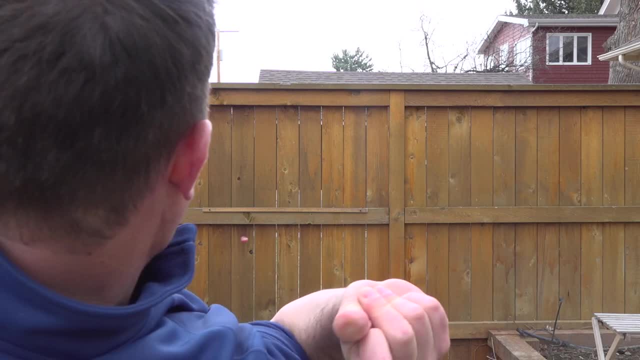 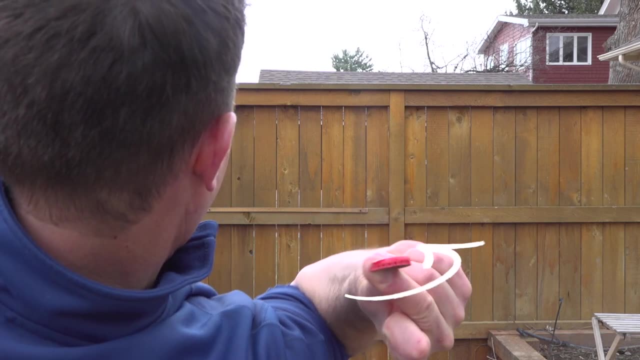 just like the last one. but once you get it down, this thing will really go and you can get to be pretty accurate with it. Physics explains why this works. We're adding energy rotational motion into that bottle cap And it would stop at the end of my finger, but Newton's first law says it will remain in motion. 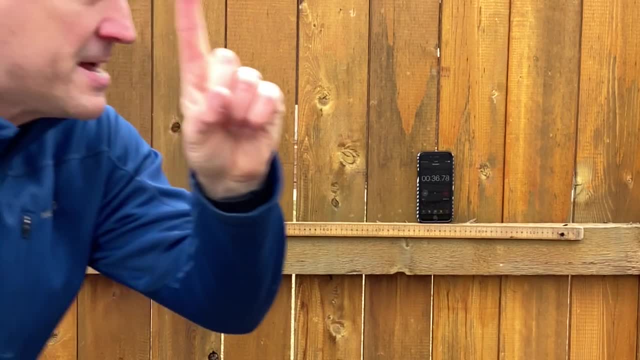 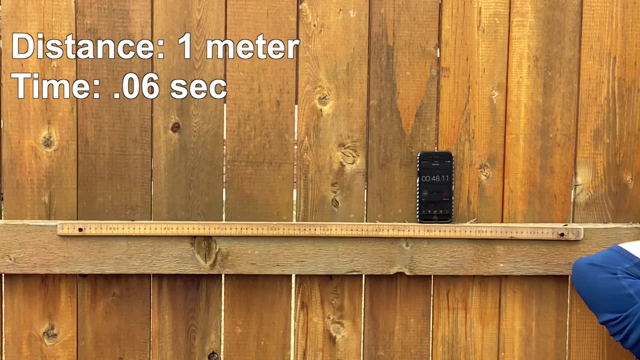 if nothing causes it to stop. Now I figured let's see if we can get this thing to fly at the same speed as the bottle cap. We got it to go about 1 meter and 0.06 seconds, That's 60 kilometers an.